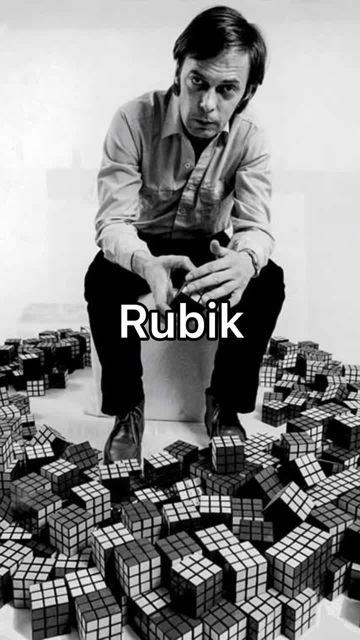 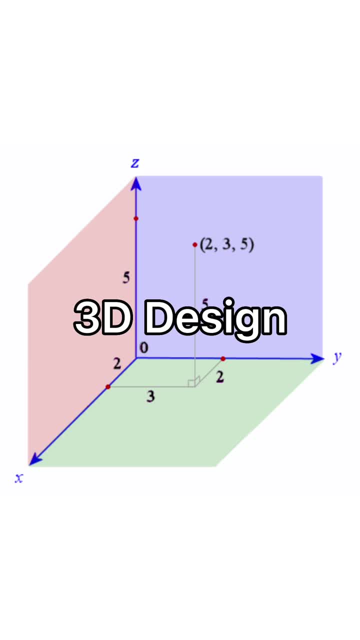 How long did it take Erno Rubik to solve the Rubik's Cube? Erno Rubik was a professor in architecture and interior design. He created the Rubik's Cube in 1974 to teach his students three-dimensional design. However, after turning the cube, he couldn't bring it back to its original state. 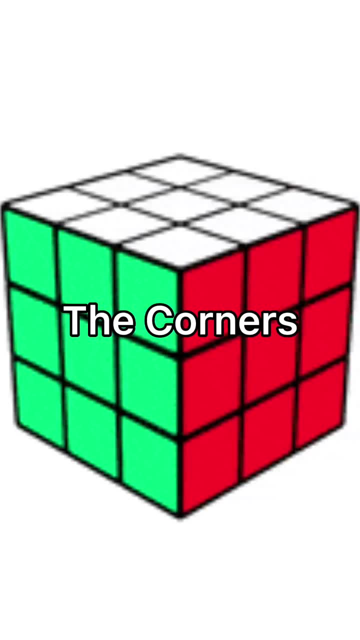 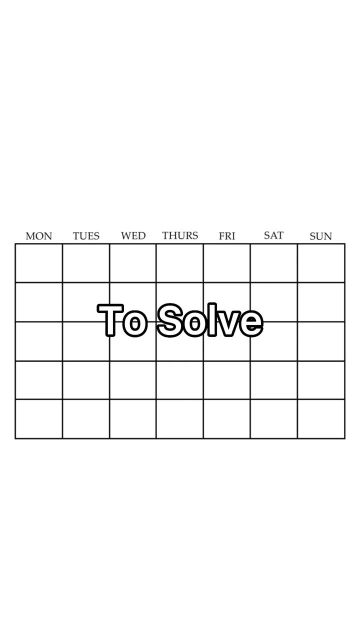 He eventually found a method to solve the cube. Rubik solved the corners of one side, then three edges, the other four corners and inserted the other edges. Overall it took him one month to solve his invention, And that is. 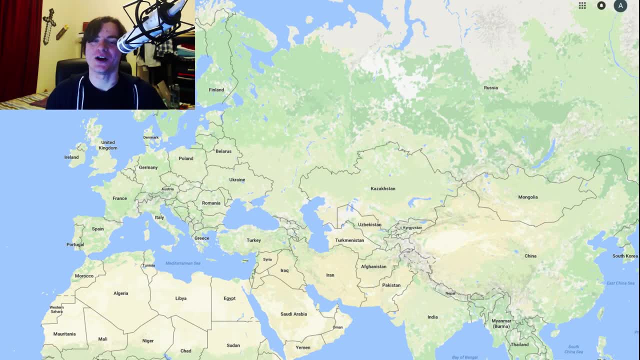 Hello, I'm a BX Toy Cat and welcome back to another second channel video. Today I have some more of Geography of the Toy Cat for you all. It's Owen's favorite second channel series where I talk about geography and the world and stuff. 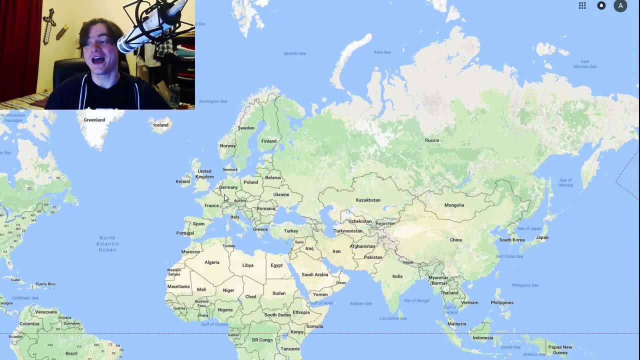 And today I want to talk about a very particular corner of the world, the one I happen to be from, and that is the continent of Europe. Well, I'm not from the whole continent, but I'm from a country which is part of the continent of Europe. 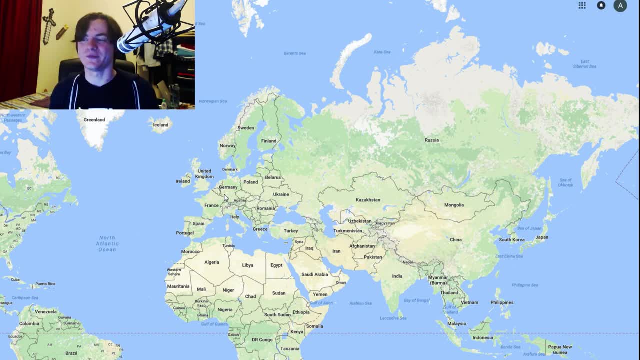 And I want to kind of talk about it today, because you often hear in the same way. you might hear someone from here say like Oh, I'd love to visit America at some point. The opposite of that is even weirder, because when you know, when you hear people from the other side of the world say like 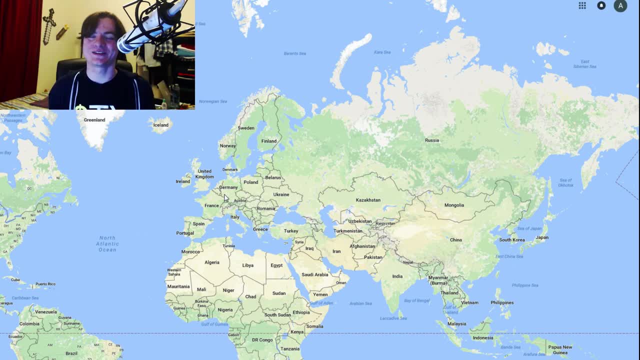 Oh, I'd love to visit Europe at some point. Or Oh, Europeans sure are crazy. Or like: Oh, European women are this or that. It's kind of a weird thing to say, because Europe is such a vast place, It is a continent. 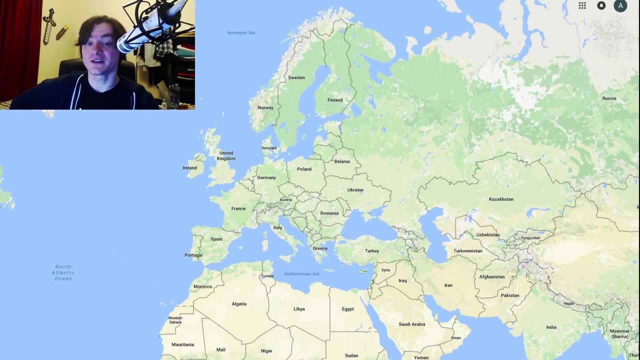 And, as a result of that, you know, when you're saying Europe, this or Europe, that you're referring to both Iceland, you're referring to the western edge of Kazakhstan and everything in between as being one whole place, which is not the case at all, obviously.